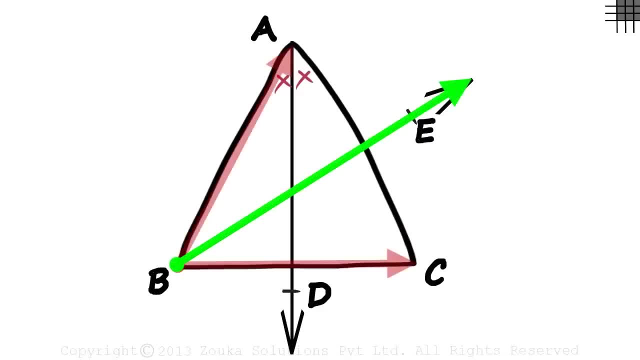 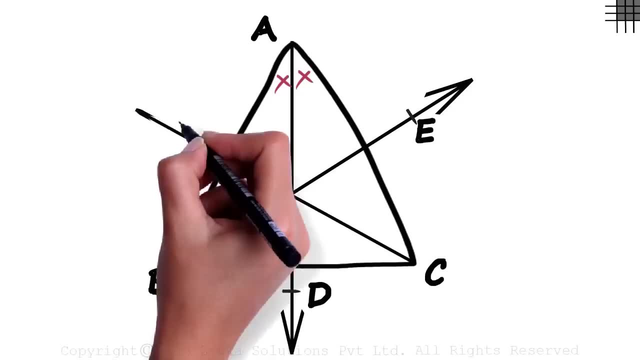 Let ray BE be the angle bisector of angle B, These two angles formed would be equal. Now we come to the interesting part. Let ray CF be the angle bisector of angle C, and that again gives us two equal angles. What's so interesting about this? 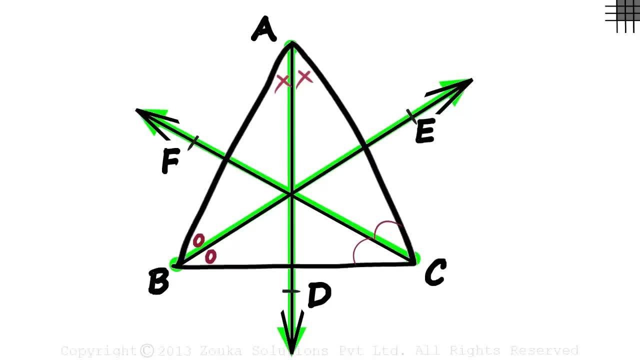 All the angle bisectors of a triangle meet at one single point. And yes, this is true for any kind of a triangle: Acute, obtuse, scalene, isosceles or whichever- The angle bisectors will always meet at one point. 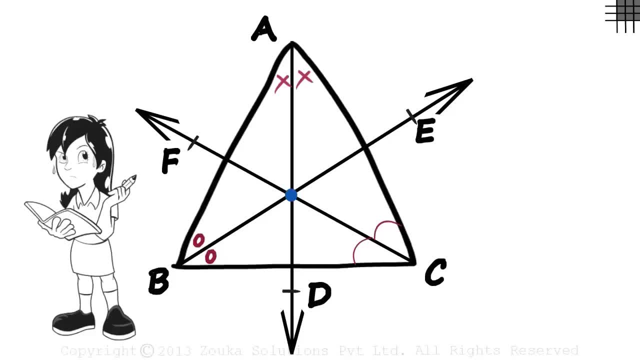 So if you are constructing angle bisectors of a triangle and you find that all of them do not meet at one point, then it means just one thing: You have gone wrong somewhere with your construction. Let's name that point I, The point where the three angle bisectors of a triangle meet. 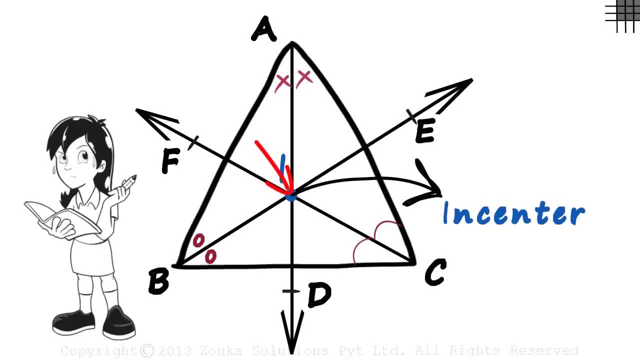 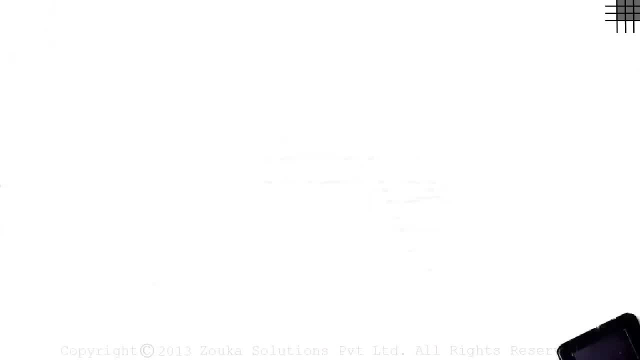 is called the in-center, But does the in-center always remain inside the triangle, irrespective of the type of the triangle? Let's erase this and look at an interesting recording. This recording is taken from mathopenrefcom and helps a great deal in understanding the location of the in-center. 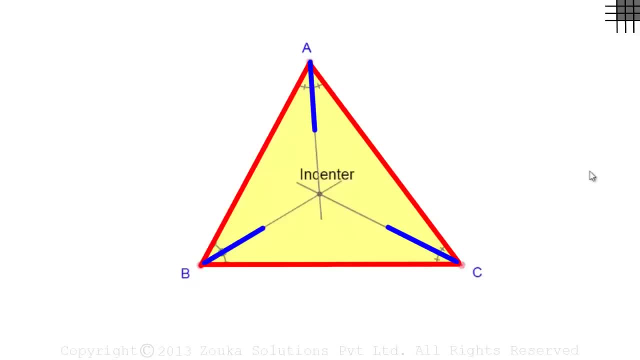 This is triangle ABC with all its angle bisectors meeting at the in-center. To understand the location of the in-center, with different kinds of triangles we can move the point A around, Doesn't matter if the triangle is acute, obtuse or right angled. 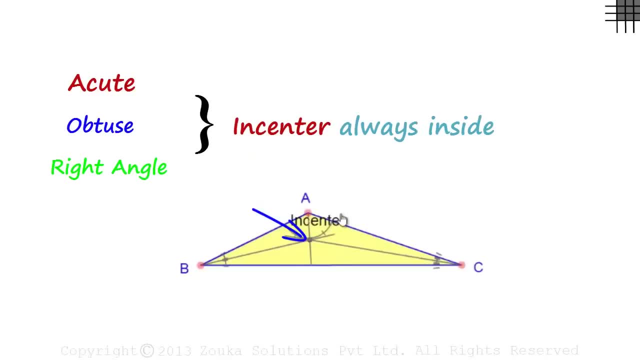 The in-center always remains inside the triangle. Even if we move point B around, the in-center will always remain inside, And the same would apply to point C. The in-center is actually a center of a circle. Where does the circle lie? 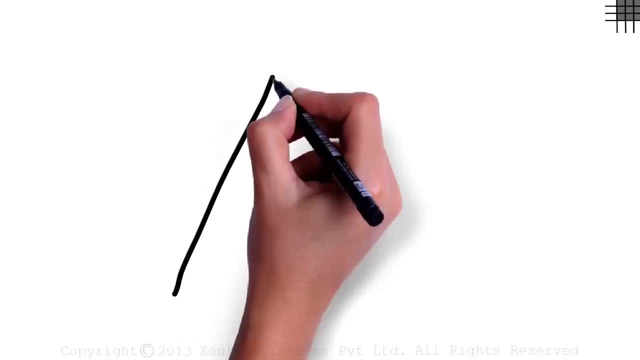 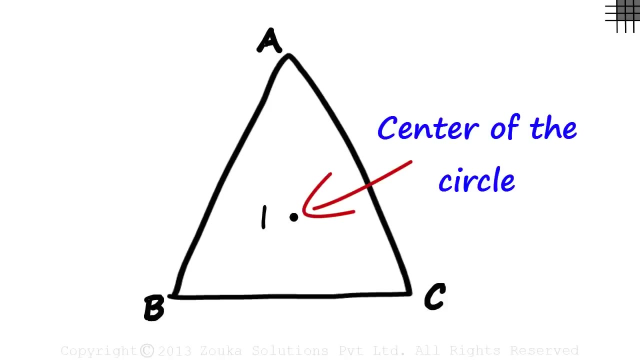 Let's see. Look at this triangle: ABC with in-center I, The point I, is actually the center of the circle, which touches all the sides at just one point. So segment AB is actually a tangent at this point. Similarly, BC and CA are tangents at this point and this point respectively.